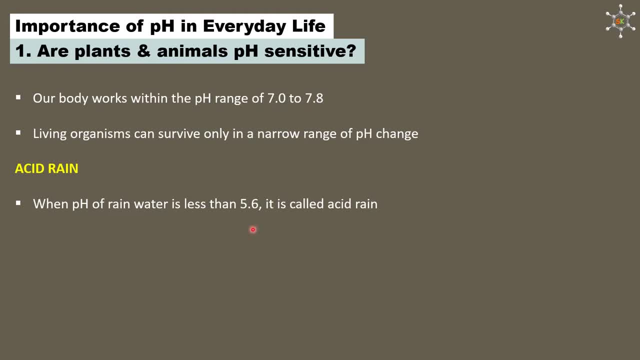 dissolution of carbon dioxide in rainwater. When acid rain flows into the river, it lowers the pH of the river water, meaning it makes the river water more acidic. Because of the increased acidic 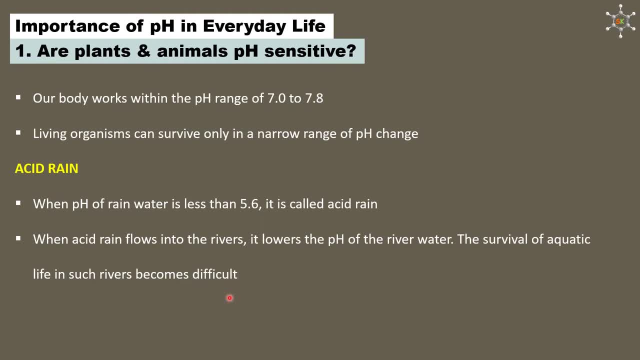 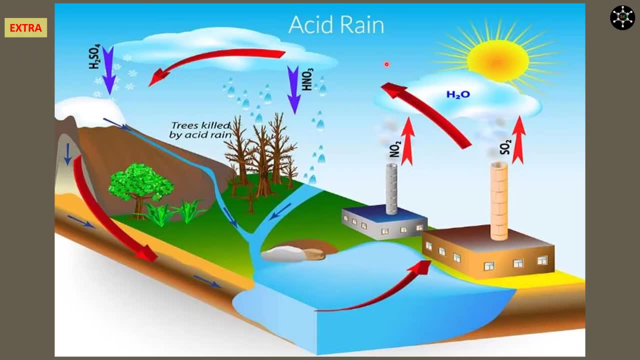 nature of river water, survival of aquatic life becomes difficult. This picture represents the addition of acids to water cycle which then comes down to earth. 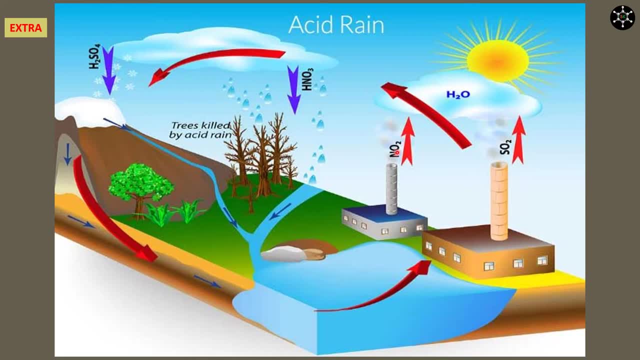 In the form of acid rain, oxides of nitrogen and sulfur which comes out as a result of industrial process reacts with water to form acids like HNO3 and sulfuric acid. These acids mix up with water and comes down in the form of acid rain which further lowers the pH of water bodies on earth. 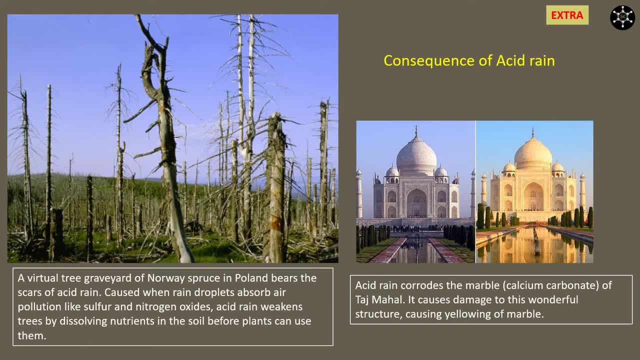 We can see the consequence of acid rain in the form of acid rain. In the first photo, trees are dead because acid rain weakens trees by dissolving nutrients in the soil before plants can use them. Second picture is about Taj Mahal. Taj Mahal is made up of marbles that is nothing but calcium carbonate. When calcium carbonate is exposed to acid which is present in acid rain, it undergoes a particular reaction. Because of that, yellowing of Taj Mahal is happening. 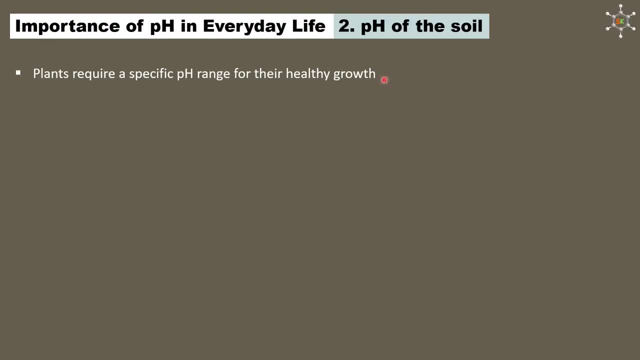 Plants require a specific pH range for their healthy growth. pH required by few crops are listed here. You can go through. 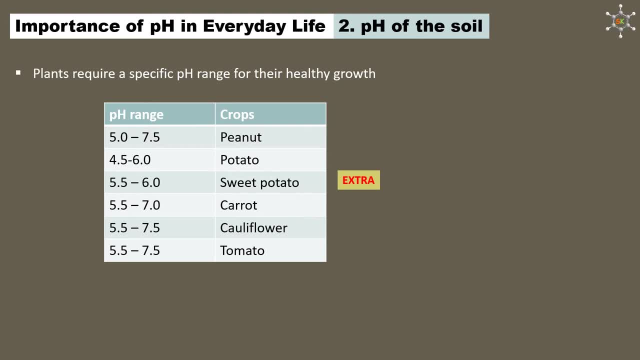 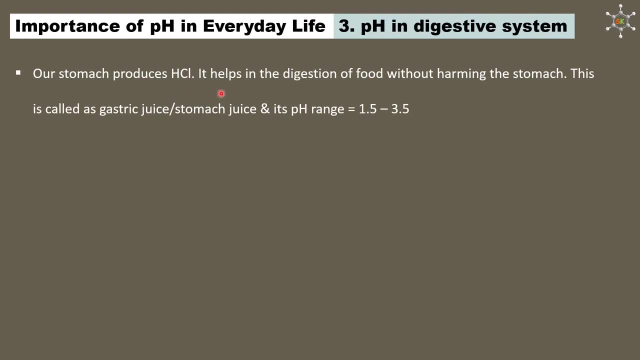 Our stomach produces HCL and it helps in the digestion of food without harming the stomach. This is called as gastric germination or gastric germination. 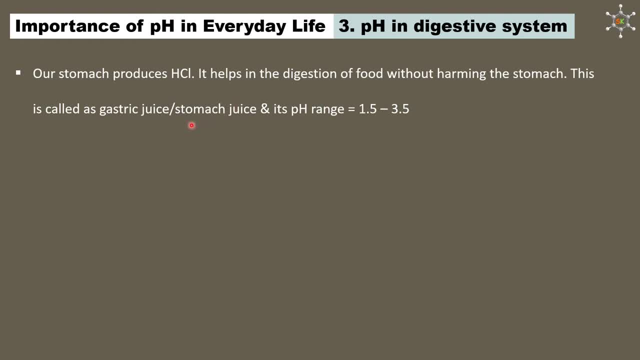 This is called as gastric germination or gastric germination. This is called as gastric germination or gastric juice or stomach juice. In Sanskrit, this is called as jatharagni. Its pH ranges from 1.5 to 3.5. During indigestion, stomach produces excess of this acid and causes pain and irritation. To get rid of this pain, people use bases called as antacids. These antacids neutralize the acid. Milk of magnesia or magnesium hydroxide is a must. One such mild base. One such mild base. 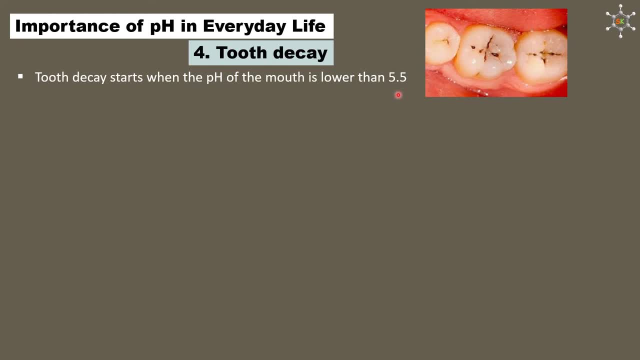 Tooth decay starts when the pH of the mouth is lower than 5.5. Tooth enamel which is made up of calcium phosphate is the hardest substance in the body. 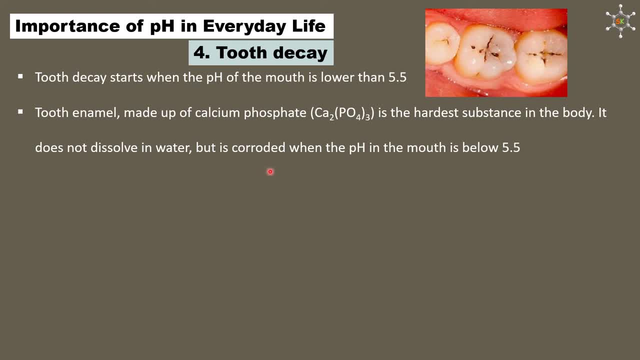 It does not dissolve in water but is corroded when the pH in the mouth is below 5.5. Bacteria which is present in the mouth produce acids by degrading sugar and food particles remaining in the mouth, and thus, the body is stuck in the mouth. 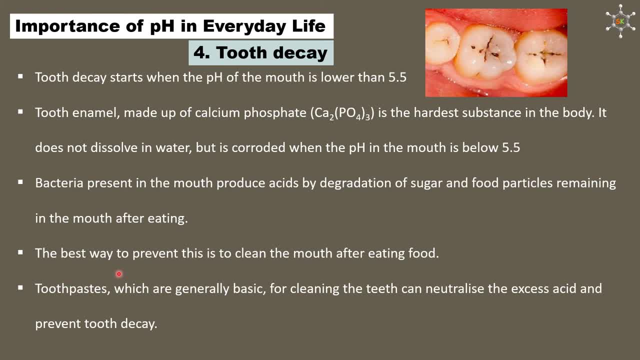 after eating. The best way to prevent this is to clean the mouth after eating food. Toothpaste which are generally basic for cleaning the teeth can neutralize the excess acid and prevent the 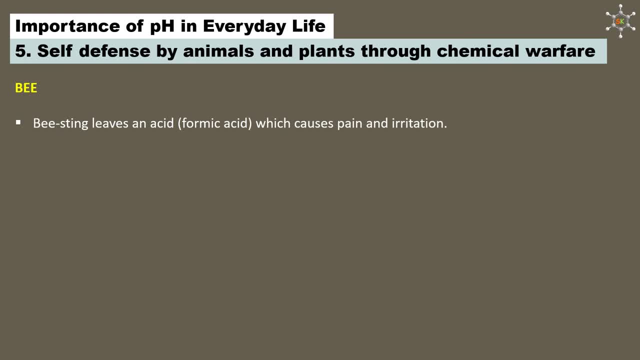 tooth decay. Bee sting leaves an acid called as formic acid which causes pain and irritation. 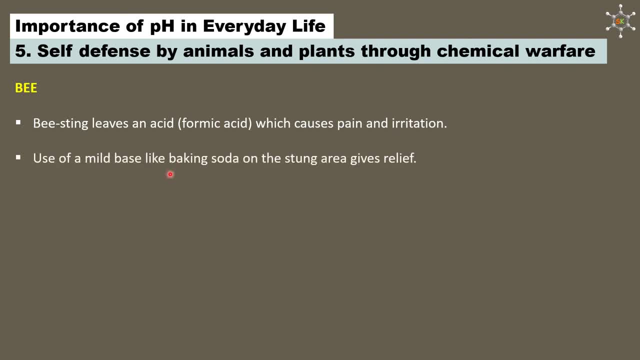 Use of a mild base like baking soda on the stung area gives relief. 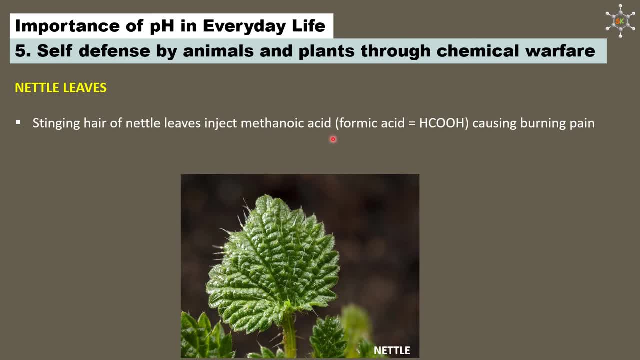 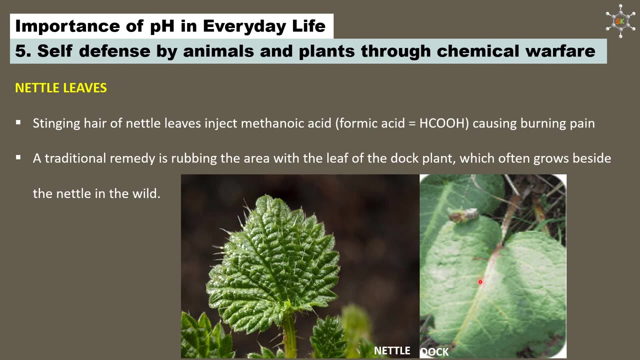 Stinging hair of nettle leaves inject methanoic acid or formic acid causing burning pain. We can see the stings of nettle leaves here. A traditional remedy for this is rubbing the area with the leaf of the dog plant. This is the dog plant. It is believed that dog plant leaves are basically used to clean the mouth after eating food. Toothpaste which are generally basic for 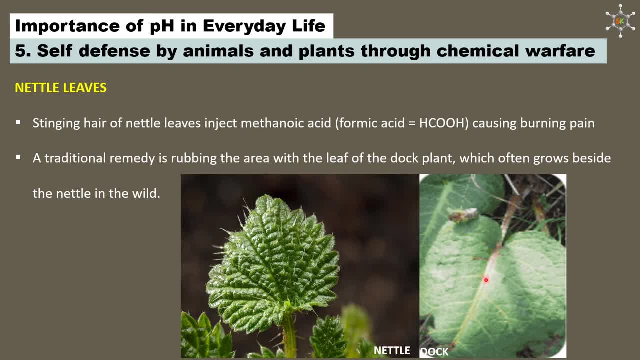 nature. It is also observed that in the wild, nettle plant and dog plant grow next to each other.